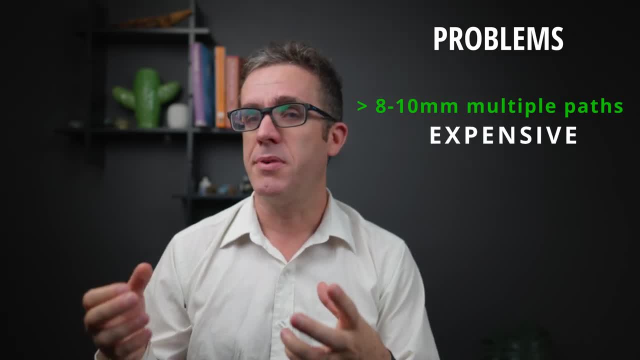 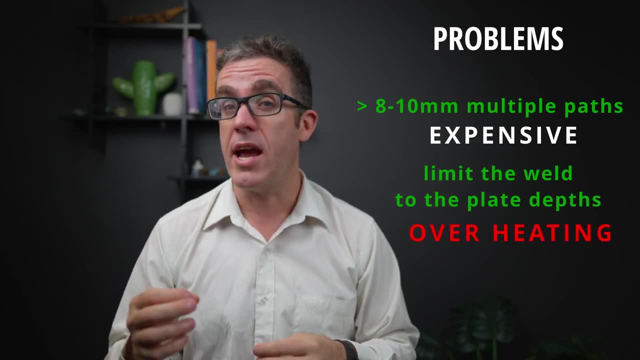 you potentially need to do it in multiple passes, So the cost can be exponential. And also you're limited by how big a fillet weld you can connect two members together, As if you go too big you can overheat the area and causing local damage, So you won't achieve the strength that 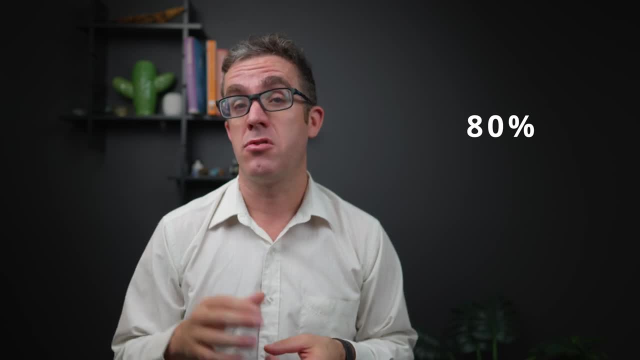 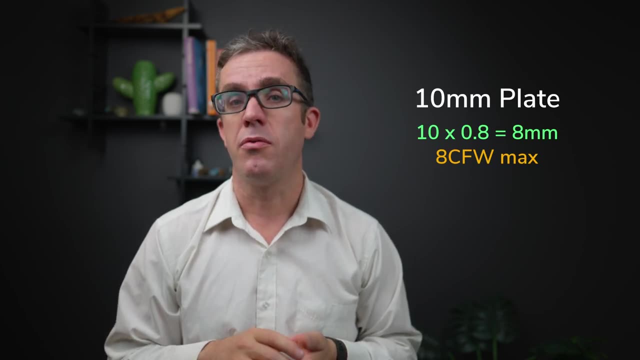 you're looking for. This is roughly about 80% of the smallest plate. So if you've got a 10 mil plate connecting to a 10 mil plate, it will need to be a maximum of an eight mil throat of the weld. Any. 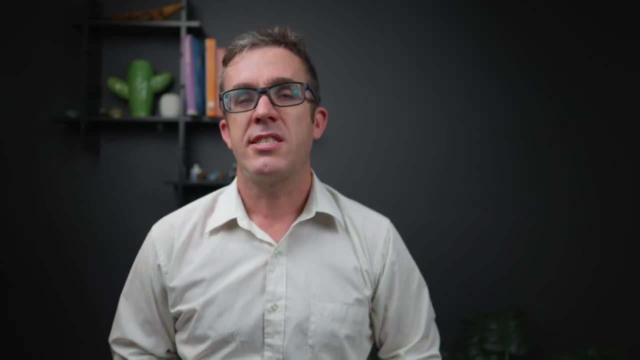 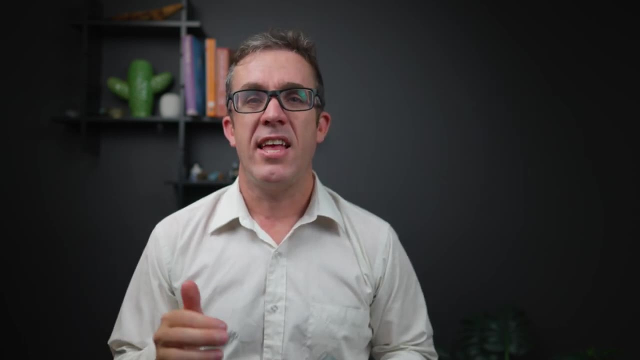 bigger and you're potentially looking at an additional damage. Much like steel, design is all about the connections. Don't forget to bolt down the like button. Not only does it help my channel out, but also allows to get this video out to more people. And, as we were saying, that welding 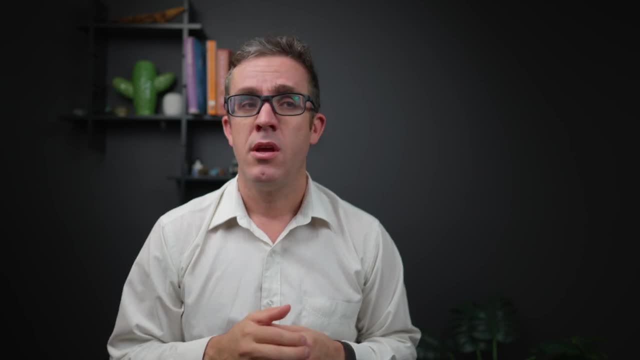 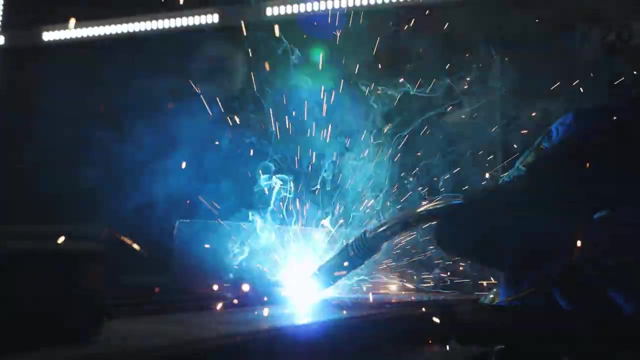 heats up the element. there's also another problem here, As we know that when we heat up steel it's expanded. So if we've got a really long section, that needs a long weld to join them together. If you just weld along them, the structural bow is essentially the steel is. 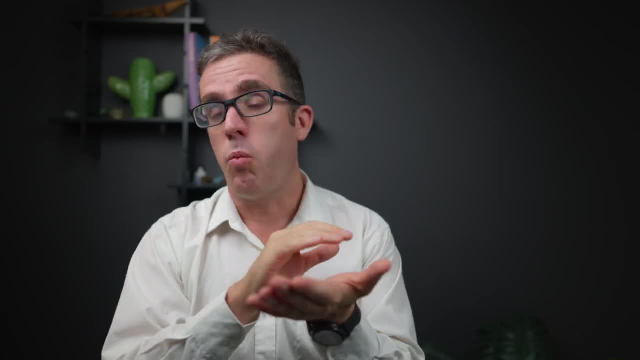 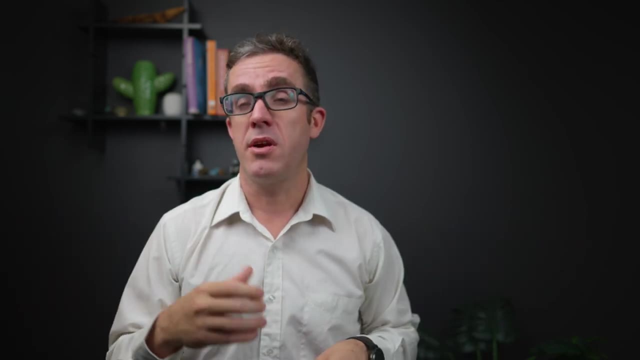 heating. in strength It's expanding And as it expands you're welding it together. You're welding in that expanded state And when it cools down it will deform and bow based on which one had expanded more as it's shrinking back to its normal state. So a way to get around. 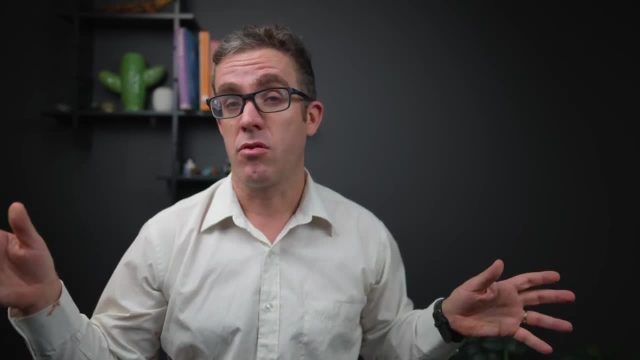 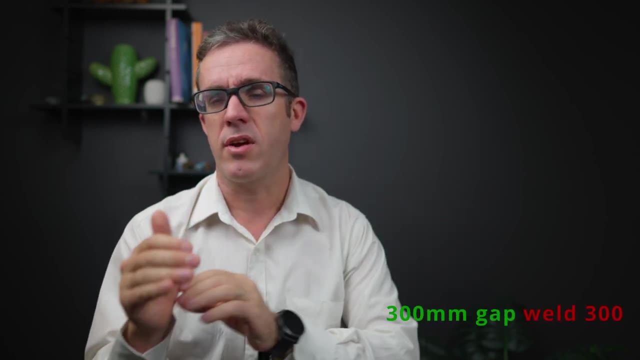 this sometimes is, if you do need to weld a member continuously along the whole section, you do it in a hit miss fashion. So you go for the first section, you might hit the first 300, then miss a 300 mil gap, hit another 300 and rinse and repeat until you weld it all the way to the end. 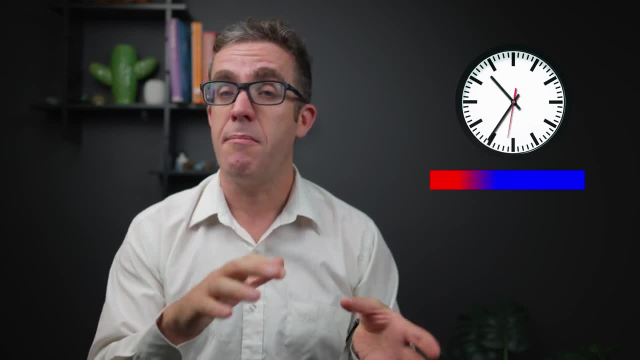 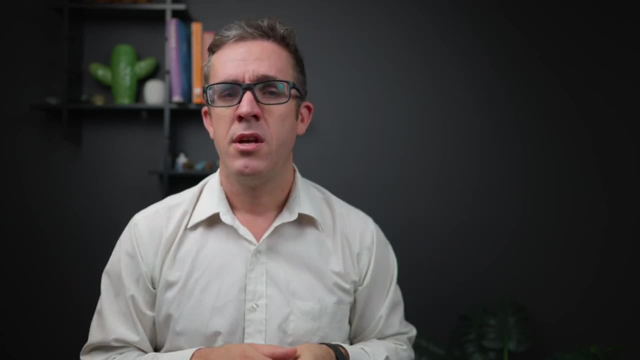 Then you wait a day or so, or even just the same day, but wait for that member to cool down. Once it's back to room temperature, you come and repeat that same process, filling in the gaps that you've created. This means you haven't overheated the element and you haven't locked in those out of. 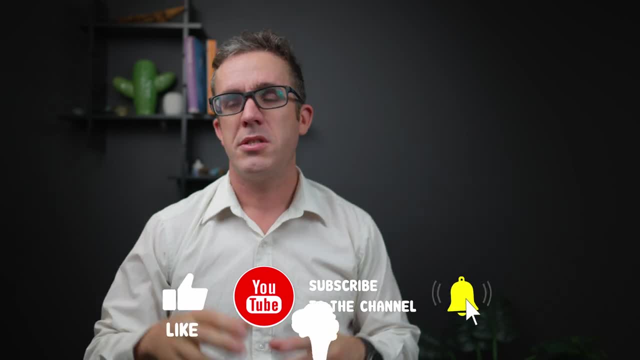 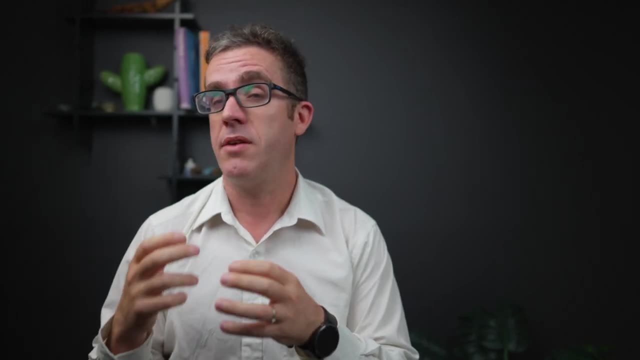 balance forces, causing the member to warp and bow. But as I was saying that welding is potentially problematic As you're taking it to site, it can get quite expensive as you need to get welders there And potentially you won't achieve the same strength as they don't have the same level of. 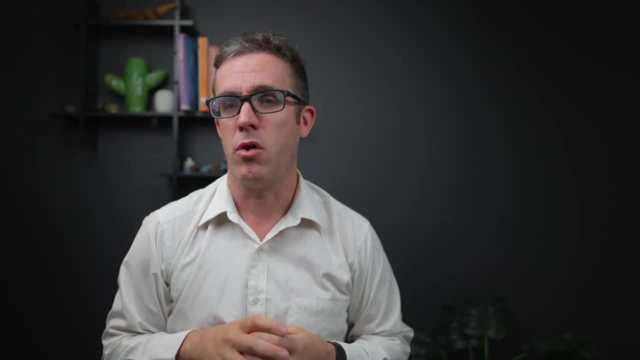 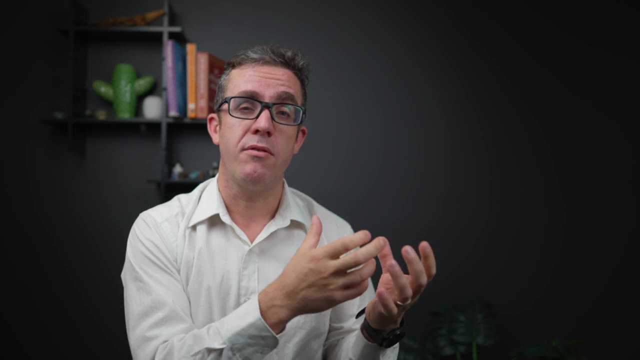 quality, as they're trying to weld up in an area which is not efficient for that welding process to occur. One of the most common methods of connecting steel structures is bolting them together, And this allows you to have the fine control that you have in the factory putting. the holes in the precise locations. You've also got manufacturer-made welding tools that you can use for welding steel structures. You've also got manufacturer-made welding tools that you can use for welding steel structures. You've also got manufacturer-made welding tools that you can use for welding. 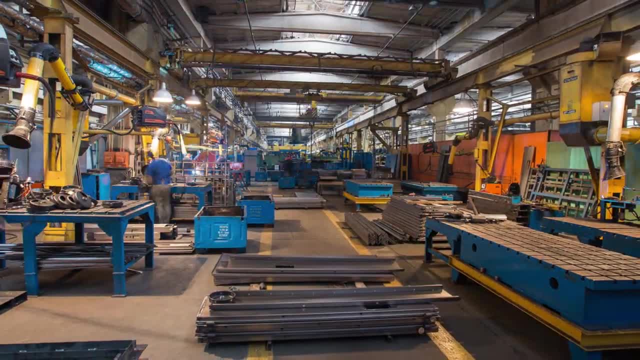 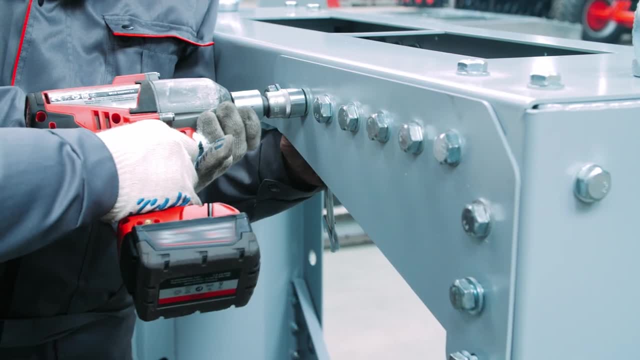 steel structures, So it'll be more interesting to integrate these bolts in a factory setting. You have high chain controls, so it'll lead to a higher duty benefit and better power generation. It's also quicker as well, potentially, sometimes, because you'll put it up and you can just bolt it together and it's already in place If you're welding something. 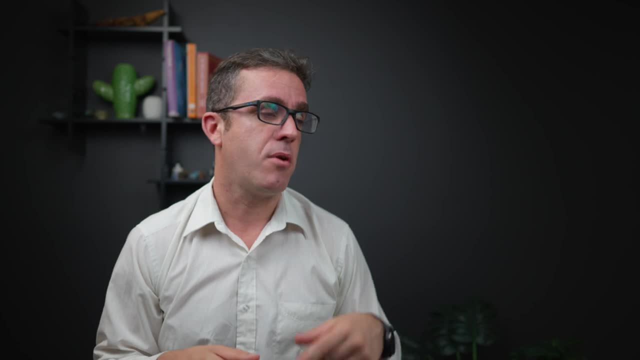 together. you might need to wait, And when we are talking about bolted connectors, they can both achieve a pinned or a moment connection. You have that versatility. There's also a number of different bolt designs for thefree hard core, So you may need to consider 4.6,. 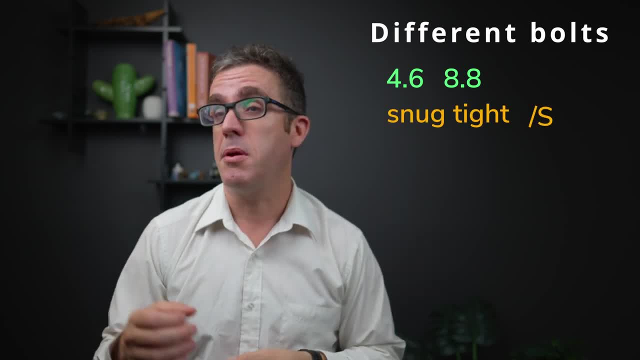 8.8 dadurch cards "-s06.. They can be Negative nighttime PROехf detail, 3ią trailer affectors, 6% of lines option. They can either be diapl celebrity solid or barrel-tight stud creatinum shield protection, Jungle T where they connect날. 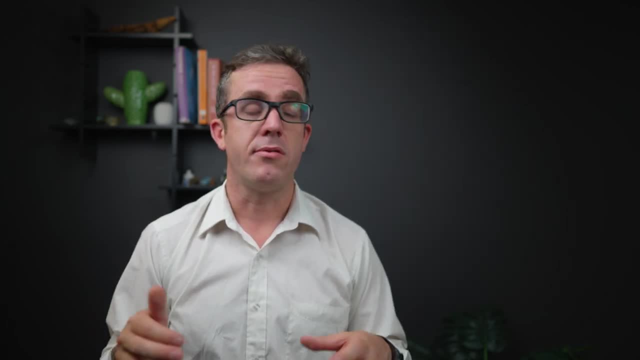 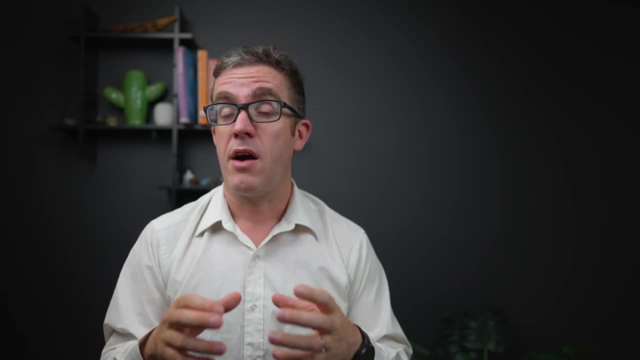 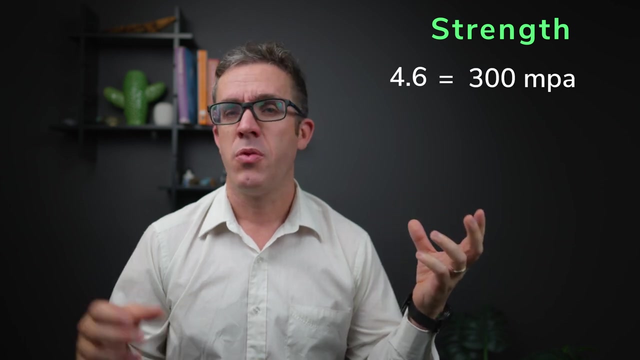 friction type, which is tf. we're talking about the different types of bolts, that 4.6 or 8.8. they both have their unique capabilities and used in their unique situations. well, first start off. the primary difference between 4.6 and 8.8 is its strength. so the 4.6 is roughly about 300 mpa. 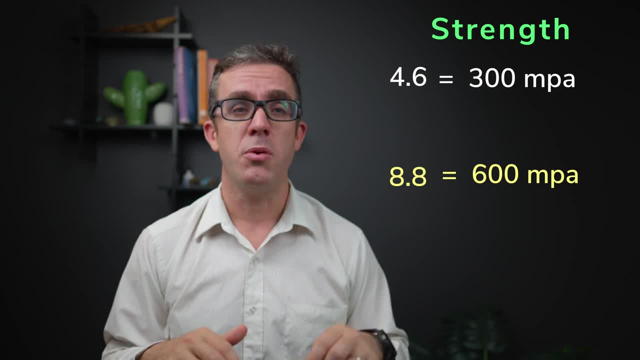 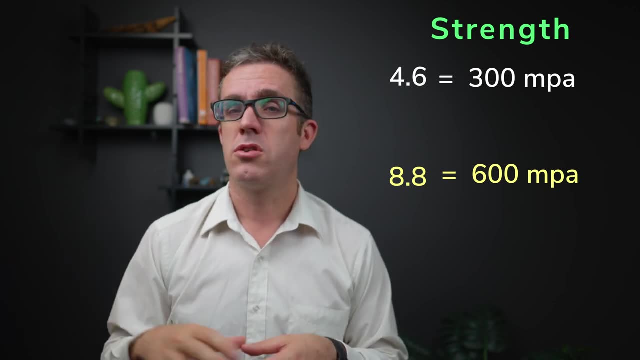 where the 8.8 is roughly around 600 mpa. so we can see with the numbers: the 4.6 is about half the strength of an 8.8. but just doesn't stop there. you just grab the higher strength ball. it's not always the for the right situation. they're also a little bit more expensive. 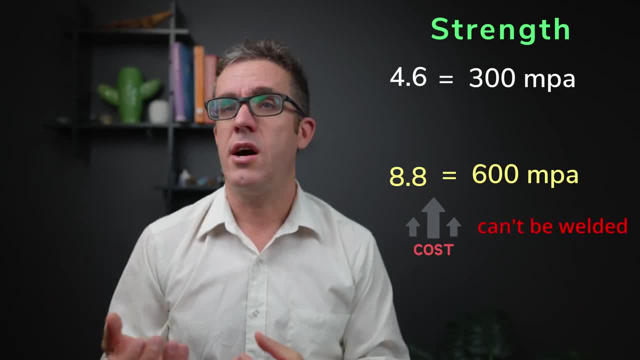 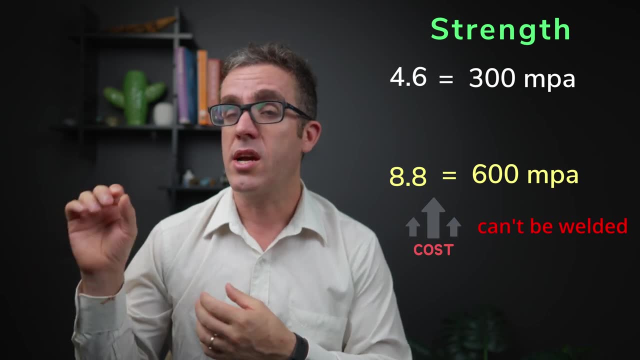 so the problem with the 8.8 is the fact that you can't weld it. it's a high strength grade of steel. if you weld it, the steel becomes brittle, so it potentially won't achieve the strength that you need. so if you're welding around it, you can't use that 8.8, where the 4.6 is a mild steel. so 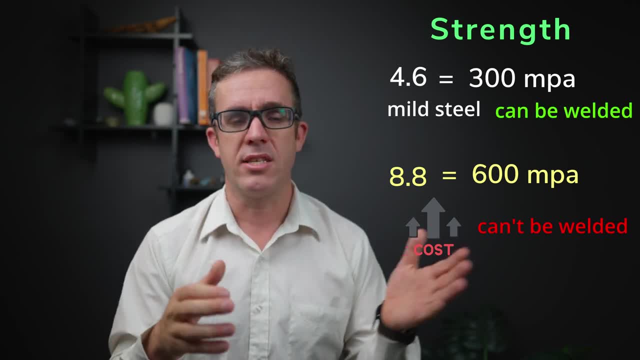 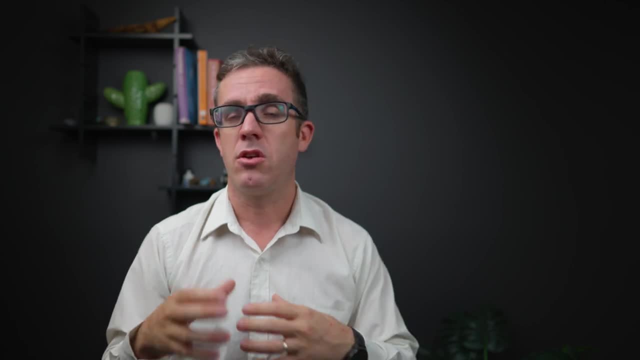 it allows you to weld it. so if you're using, in situations such as welded studs for whatever reason, you can't bolt all the way through and you need a welded stud there, you can bolt it on and have it with a 4.6 if you've got members that don't need that high strength. 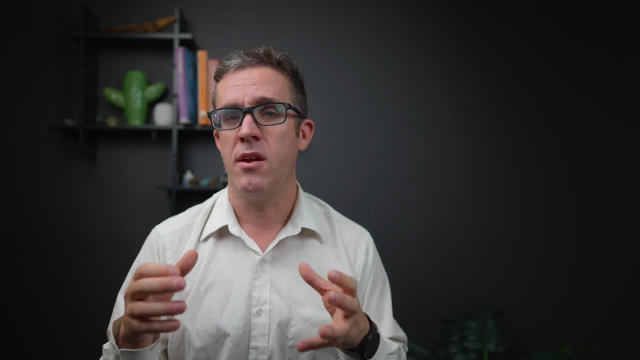 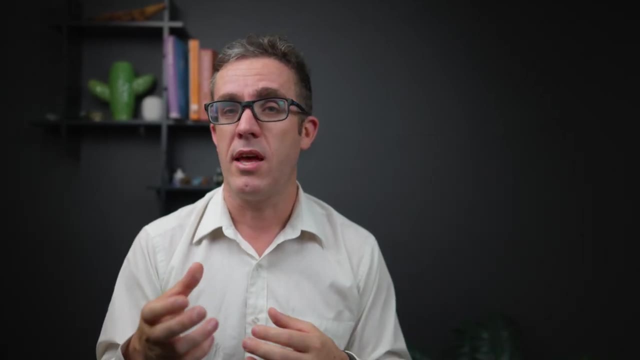 such as bolting to timber or to purlins, so they don't have really big moment capacities or loads that they need to resist. the 4.6 is better. it's a little bit more versatile, you don't need to worry about that overheating issue and it's cheaper. well, typically if you're connecting. 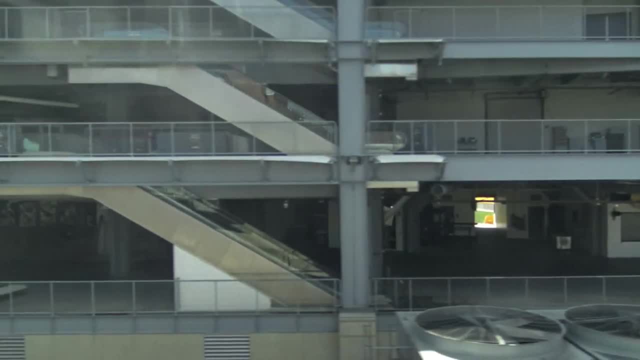 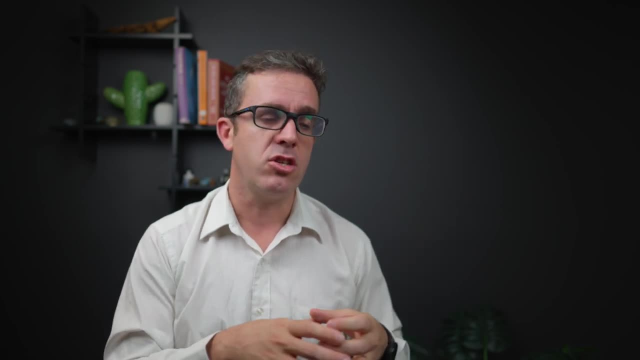 steel to steel connections, you need to make sure it achieves the exact strength that 8.8 is typically used for steel beam or steel column connections. 4.6 on the other end, as you can weld it, it allows you to place bolts more precisely. so, for whatever reason, you've got tying down bolts and you want. 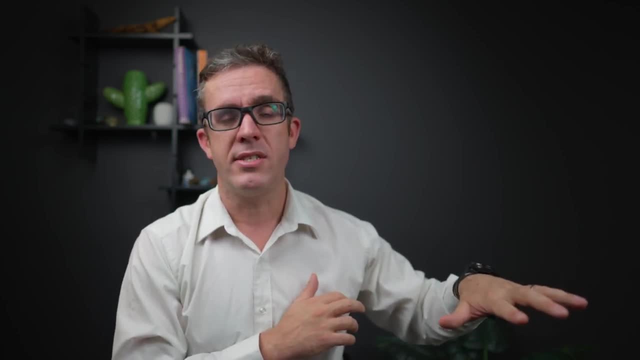 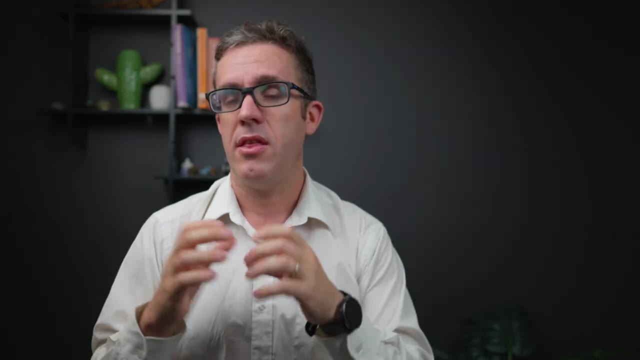 to make sure the template is accurate. typically you use that 4.6 in the tying down bolt situation. spacing of bolts is super critical when you're looking at how you're detailing your connections. there's a number of rules that you have to abide by to spacing those bolts out in the correct locations. first up is spacing them enough. 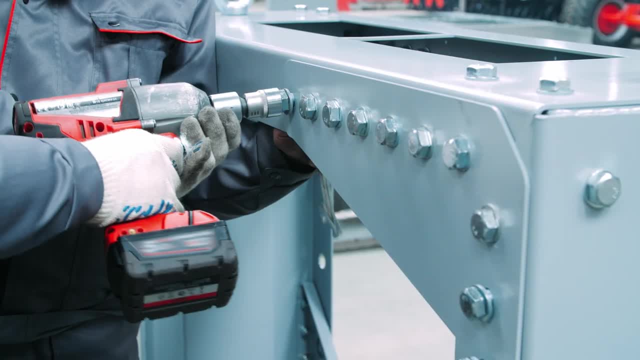 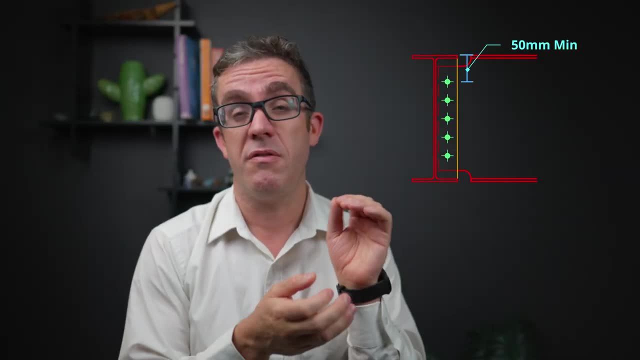 so it allows for the installation to occur. so if we've got the bolt there, we also need to put a ratchet gun or socket over the top. so we need to make sure we've got enough distance around it. we need to make sure they've got at least 55 to 65 clear of any flat plates to allow the ratchet gun. 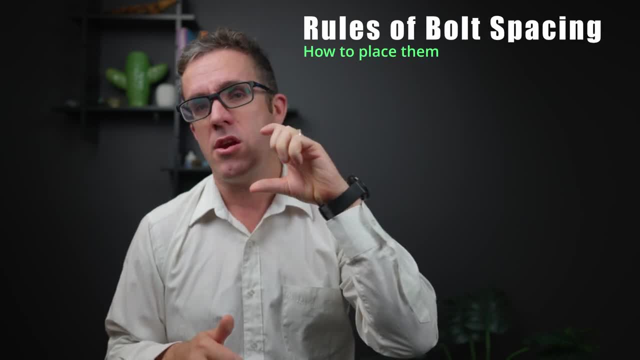 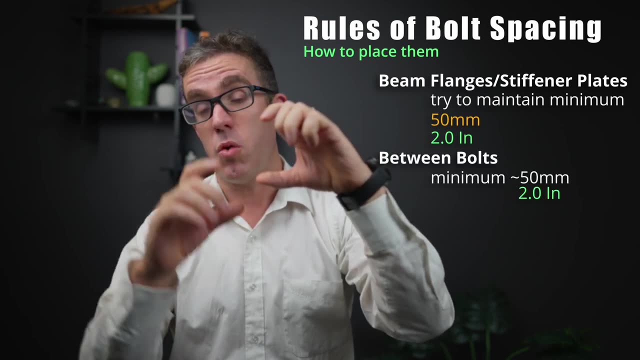 an above tip or vice versa, to achieve the torque that we need. the other concern as well is that make sure that you've got enough gap between those two bolts. so typically when you're spacing out your bolts, you'll make sure there's at least 50 mil clear between each of the bolts. that is your bare. 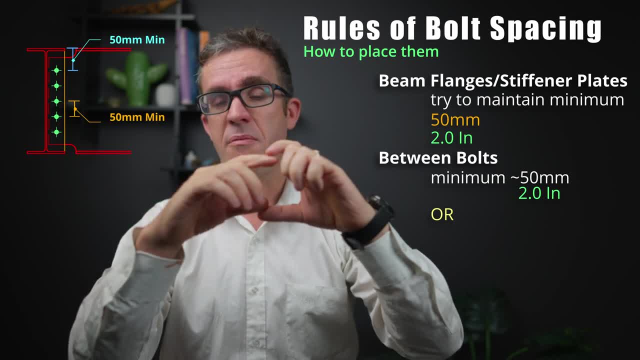 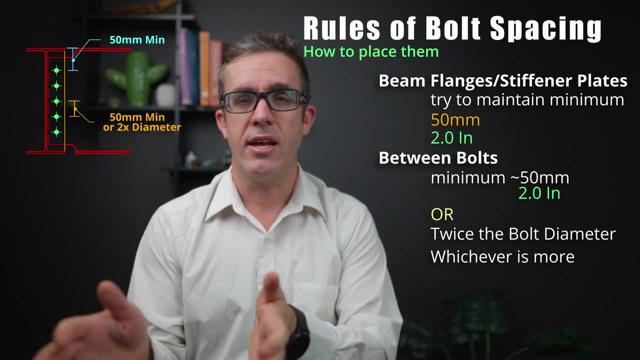 minimum. that's for your smaller type bolts. but when your bolts start to go up in size, you need to have a bigger and bigger gap, which is roughly about two times the bolt diameter. the reason for this is it needs to transfer shear through that connection. so you need to make sure. 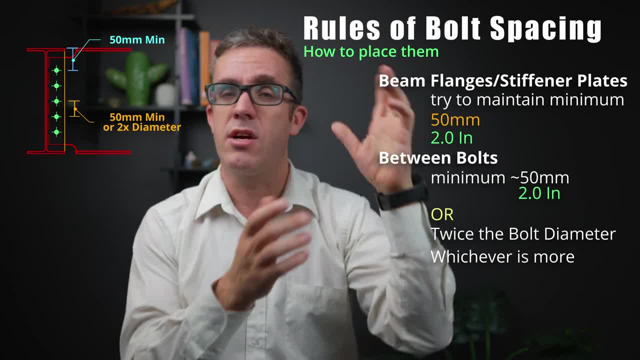 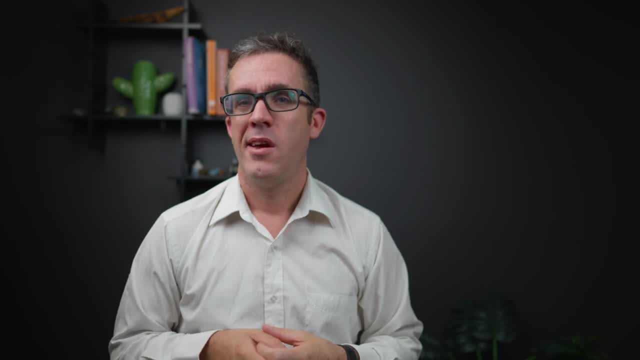 you've got enough steel, after you take out all those holes, to transfer the shear that that connection is trying to transfer through the chain unit back and forth back to the structure. as we're saying, there's really two types of connections you can have. we'll first go through the moment connection. now a moment connection that's bolted together can 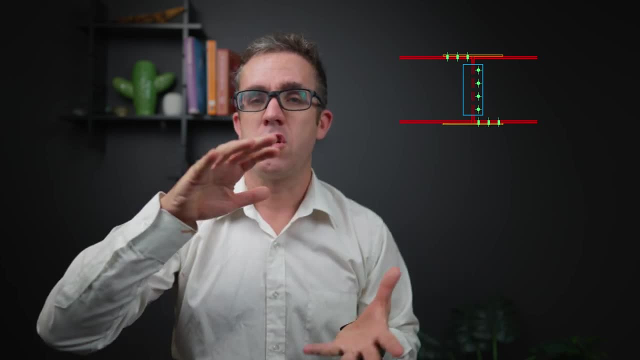 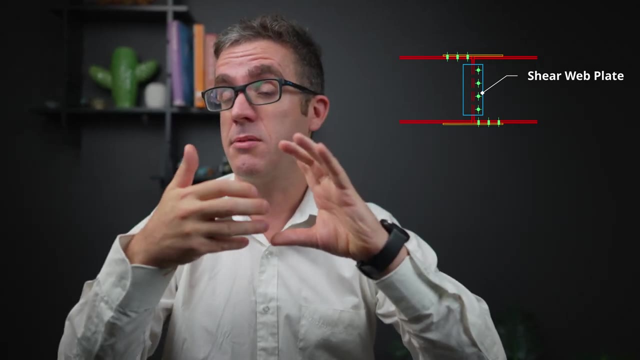 either come in two forms. the first one is where we've just got shear plates and top and bottom plates. now these plates have different functions, so we've got the central. web plate is where you get most of the shear transfer, and that's similar to when you're designing a steel beam. so you have 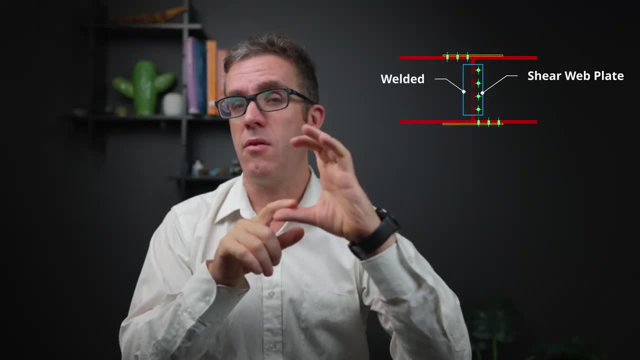 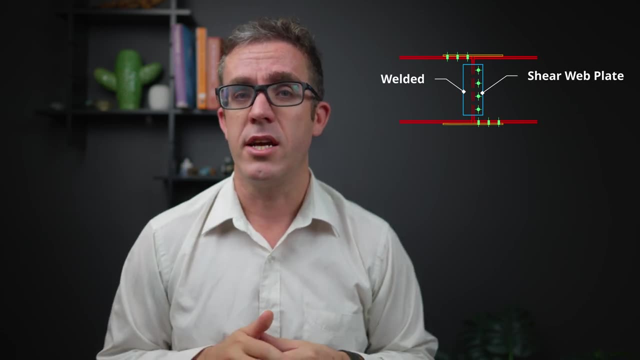 your central steel plate that'll be typically welded on one side to limit the amount of work you need to do and bolted on the other. the purpose of this central cleat plate is only to transfer the shear in the location. the critical nature of this single plate onto the web is really there. 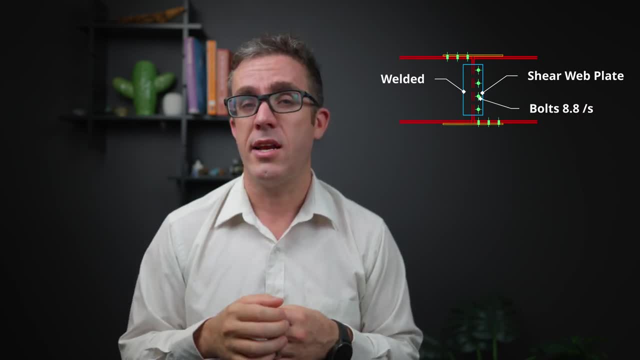 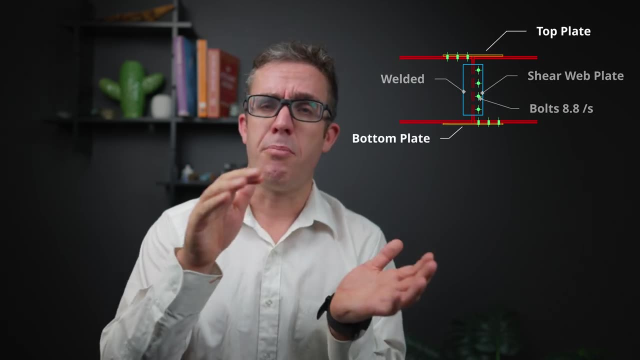 just to transfer shear. so typically you only need to make the bolts snug tight as you don't mind a little bit of movement in them. but it allows for that shear transfer similar to what you do in steel beam design where if the top and bottom plates you're bolting through the connection. 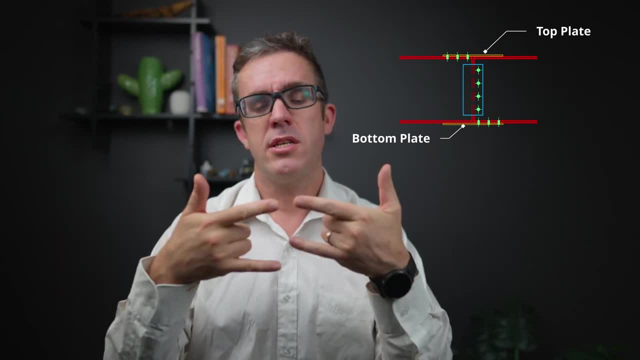 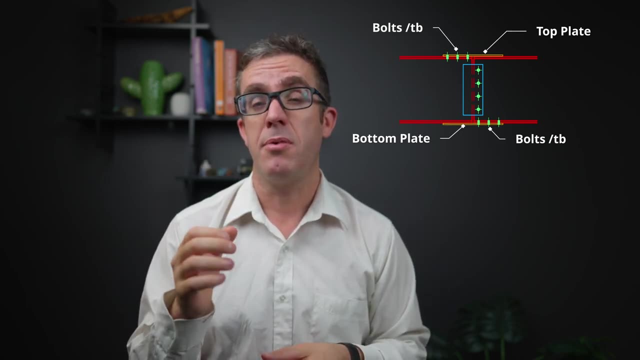 and that's allowing for the transfer, the compression or tension force. this is really for your moment fixity. so the top and bottom plates need to transfer those high forces and typically you will have tb bolts there, as you wanted to grab a little bit earlier so we can have a more stiffer connection as a softer. 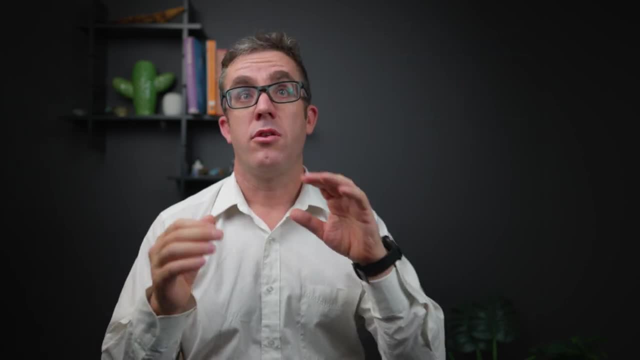 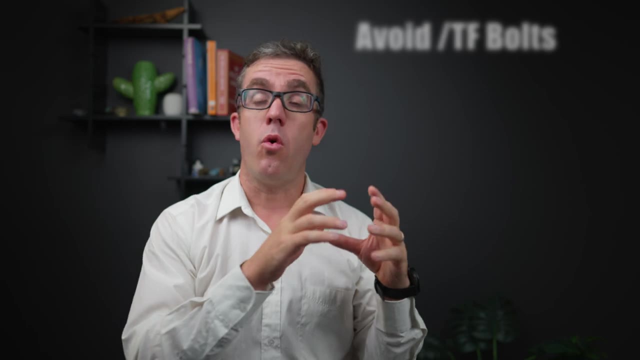 connection there may be a little bit flexible. talking about tb bolts on the top and bottom of the plates, there's also another one that we talked about, which is tf, which is friction type bolts. typically you try and limit or try to not need friction type bolts wherever possible. it's a 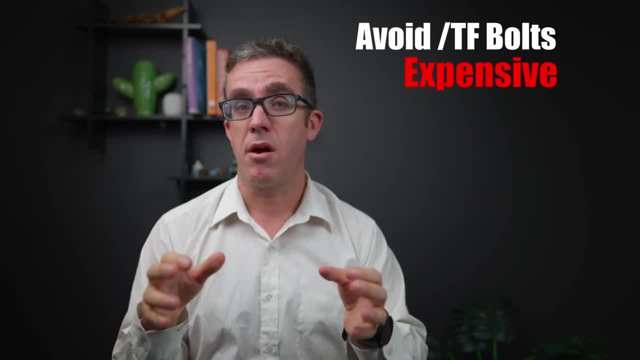 really expensive connection. essentially you need to roughen the surface, you need to prep it. also the bolts need to be torqued at a high altitude, so you need to have a really good connection load. so not only is it more expensive due to all the preparation action, i mean they have a lesser. 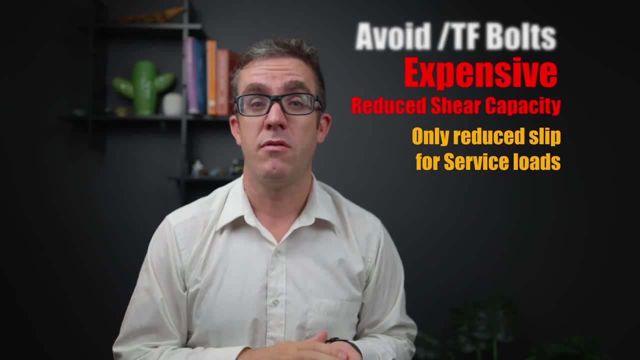 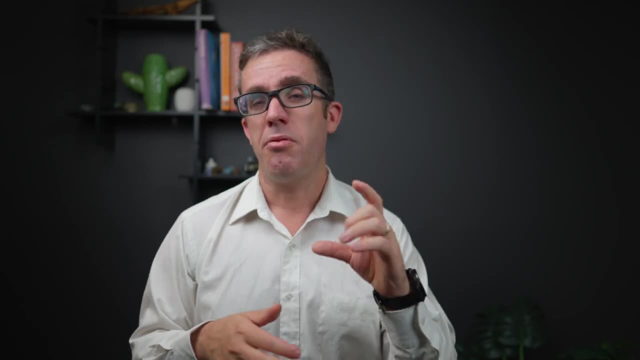 capacity to resist shear. that slip is only there for service moment. it doesn't limit slip in an ultimate situation. so you only put this in situations where it's highly sensitive to movement. one pro tip: when you are putting those connections in, the ones on the side plate are 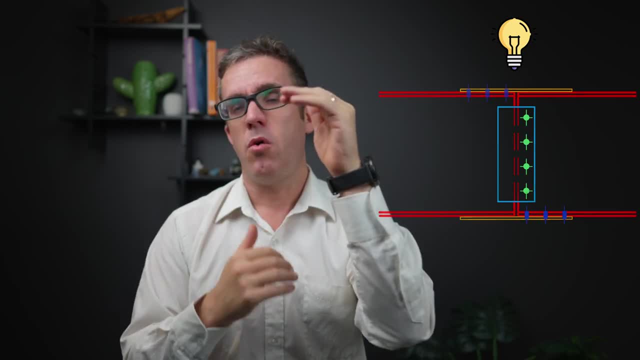 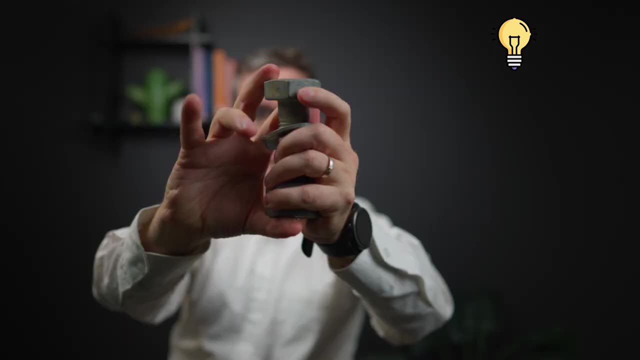 quite easy. you can put them either direction, but the ones on top and bottom always make sure that the nut is on the bottom. the reason for this is, if it ever becomes loose, you'll still have the bolt. you can come back and bolt it up later, where, if it's up the other way, the bolt will fall through. 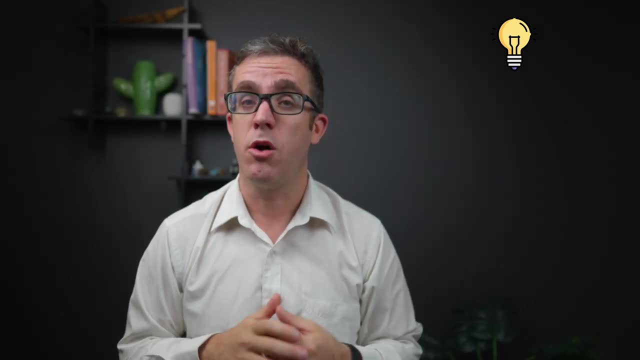 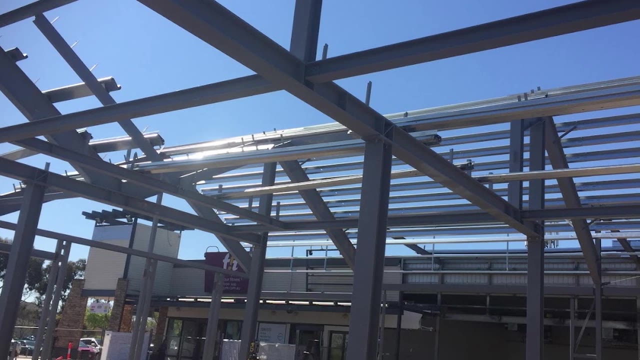 you'll have the nut resting on top, and the nut resting on top really doesn't help you at all. the next type of connection is an end plate connection. these occur in a number of different locations, so you can either have this budding up towards a column. you can either have this: 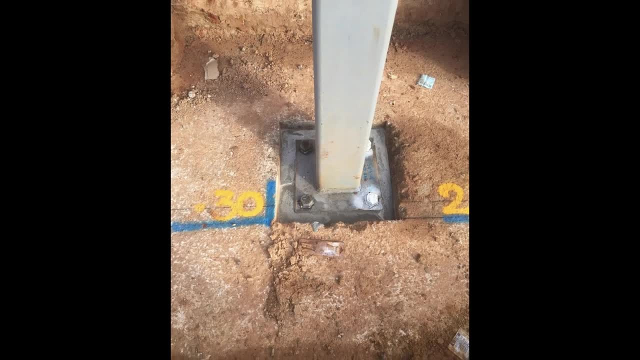 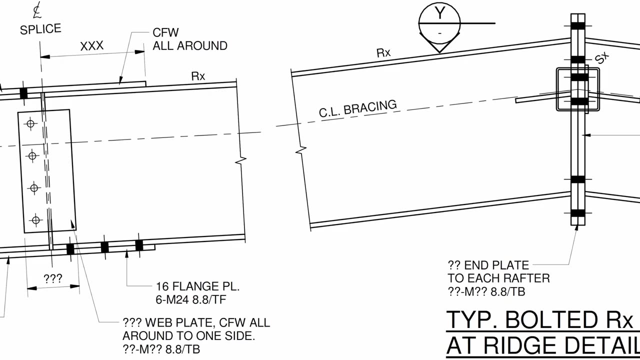 budding up towards the wall, or you can have this as a base plate, so there's a number of different situations that you can put them in, depending on the stiffness of your plate. will depend on whether that's a moment connection or a fixed connection. typically of thicker plates allow for less movement. 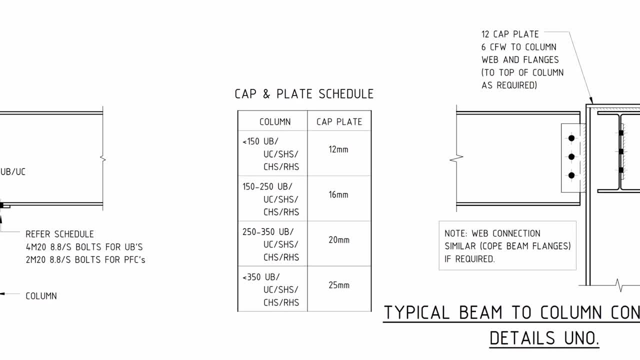 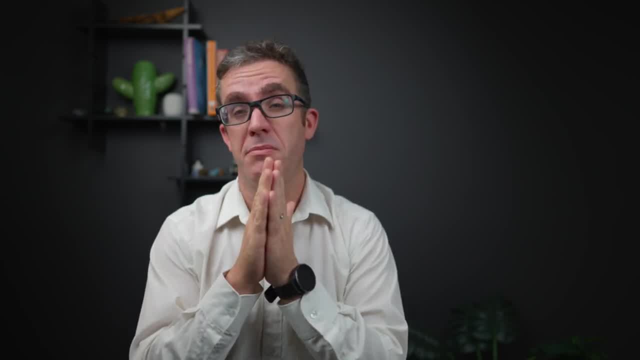 so you don't provide the fixity where, if you just need it for a base plate such as a column, you want to make sure your base plate isn't too thick. so you don't provide the fixity that you may not be looking for with these type of connections, or whether you're just beam to beam, beam to column. 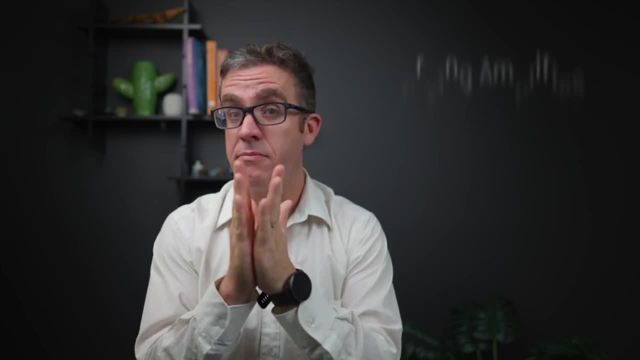 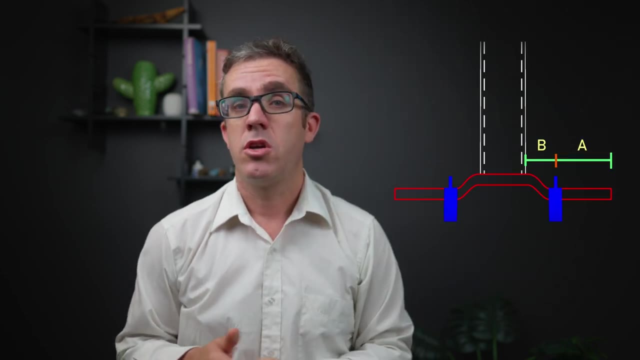 or even on that slab. potentially there's a problem with prying, which is an amplification of the force. so there's a number of ways that you can deal with this. first up is trying to increase that a to b ratio to at least 0.75, to make sure that a is smaller than the b, to make sure you're not. 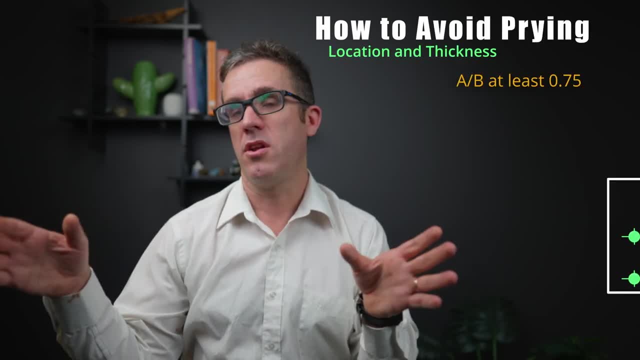 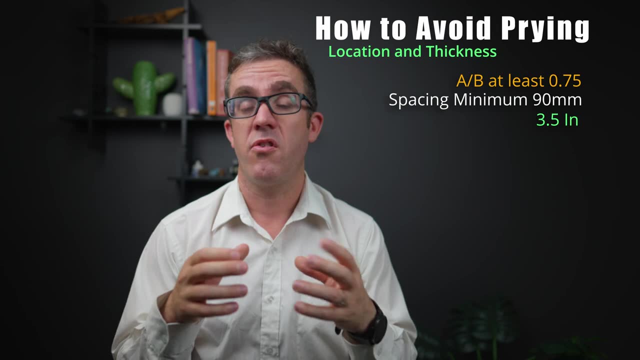 getting those prying actions that occur. sure you're at least spacing your bolts more than 90 millimeters apart to make sure they're not too close to cause that coupling action to occur. and next one is also making sure the thickness of your base plate is thick enough. so if you've got a really thin base plate it can cause those prying.